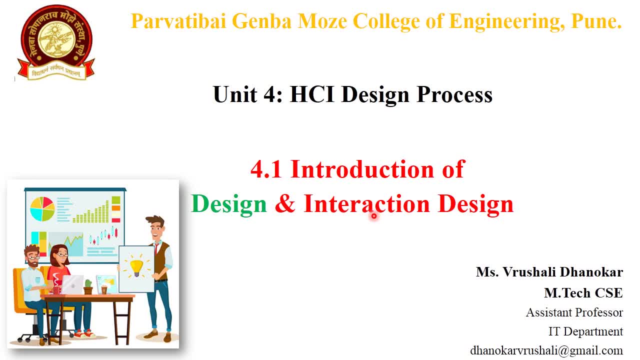 Hope you have watched my all previous videos. Now, from in this session, we will start our 4th unit, that is, HCI Design Process, And the first unit in this point is Introduction of Design and Interaction Design. In this video I will give you just introduction about Interaction Design. 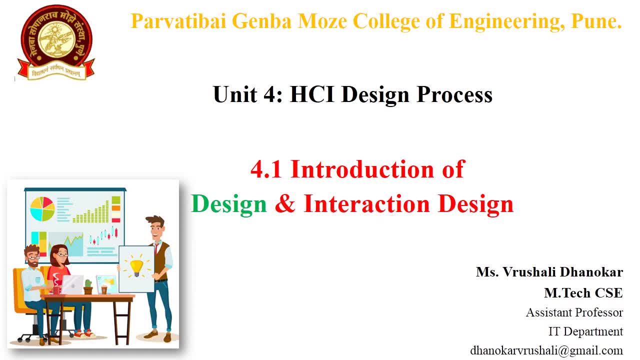 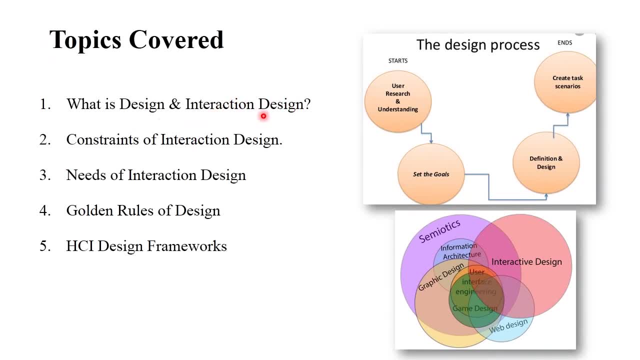 So let's see what is meant by Interaction Design. Next Coming points are covered in this video, which includes: what is Design and Interaction Design, Constraints of Interaction Design, Needs of Interaction Design, Golden Rules of Design and some HCI Design Framework. 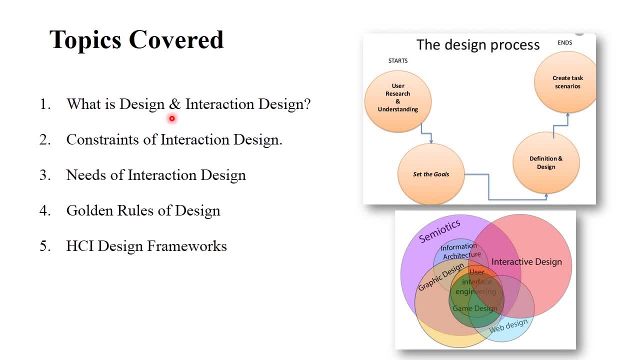 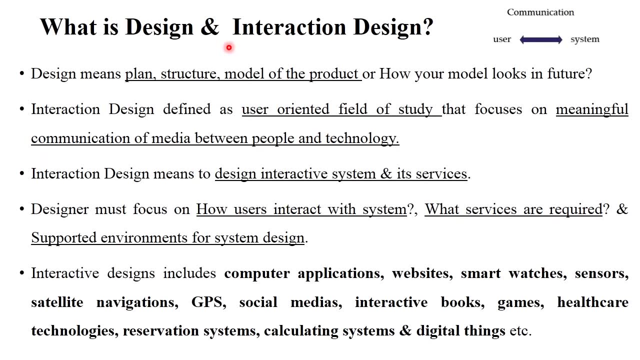 So let's see one by one. The first point is: what is Design and Interaction Design? Next, So what is Design and Interaction Design in Human-Computer Interaction? In my last videos we learned about Interaction Design and some introductory part about that. 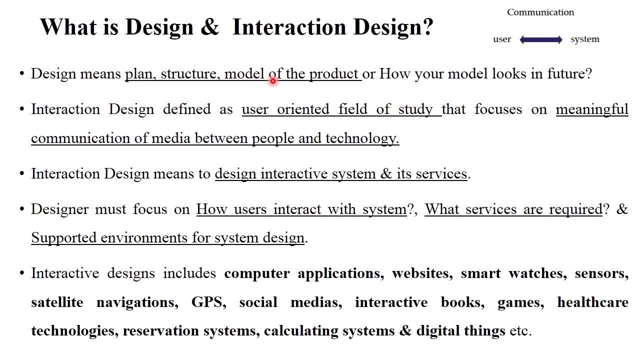 So Design means Plan, Structure, Model of the particular product, or how your model looks like in future. This is called as Design And Interaction Design, defined as user-oriented field of study that focus on meaningful communication of media between people and the technology. 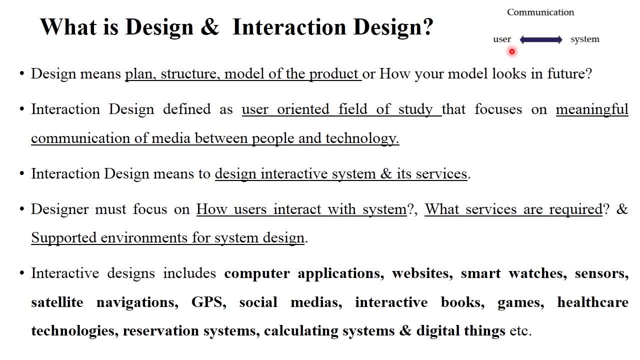 So Interaction Design simply means the communication between user and the system. right Interaction Design means to derive interactive, interactive thoughts from the system and its services. Designer must focus on How user interact with the system, What services are required and Supported environments for System Design. 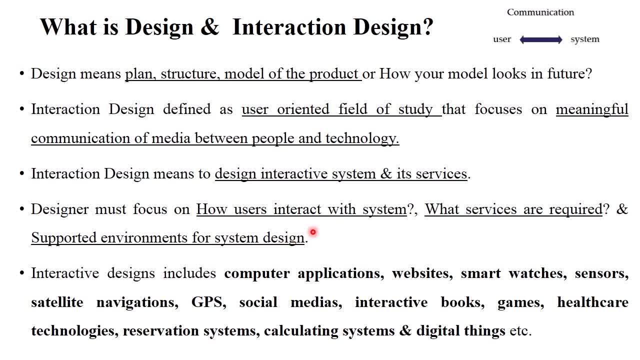 I will give you one example, For example, Whatsapp. We all are familiar with all the social medias, So Whatsapp is most interactively designed, right? So developer thinks that which types of services are provided to the user, That is, chatting applications, video call, audio call and some other activities. So developer thinks that what is the most interactive And how to interact with a user. So developer thinks that which types of services are provided to the user, That is, chatting applications, video call, audio call and some other things. 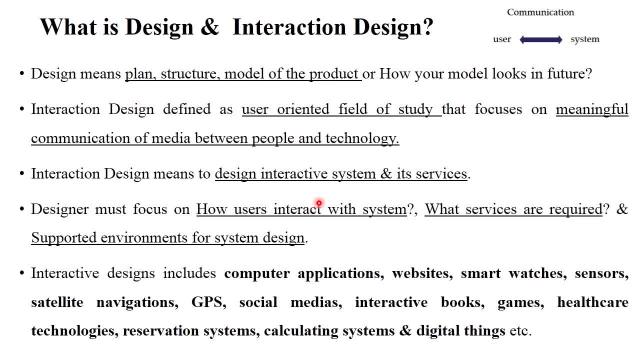 other applications or services also. so user interact with the whatsapp or other social medias and use those app as per the requirement, right. so interactive design includes computer applications, websites, smart watches, sensors, satellite navigations, gps, social medias. some interactive books are available online, then games, healthcare technologies, reservation system, calculating. 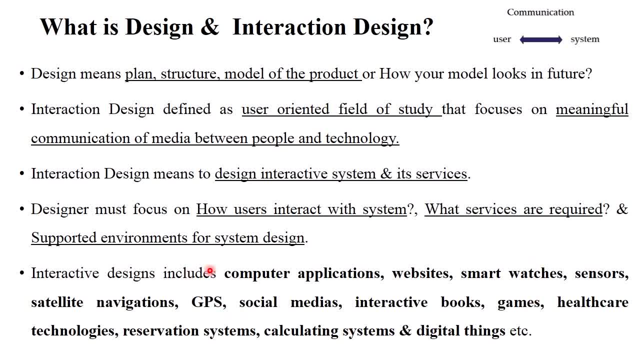 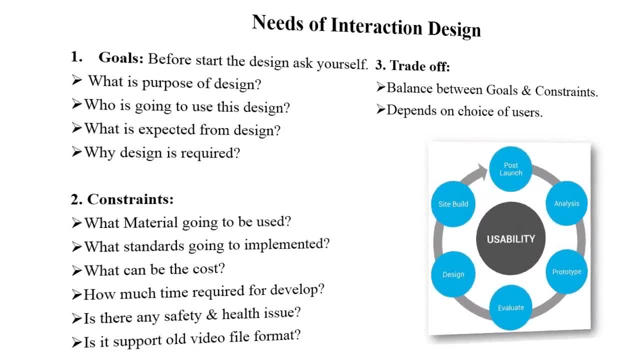 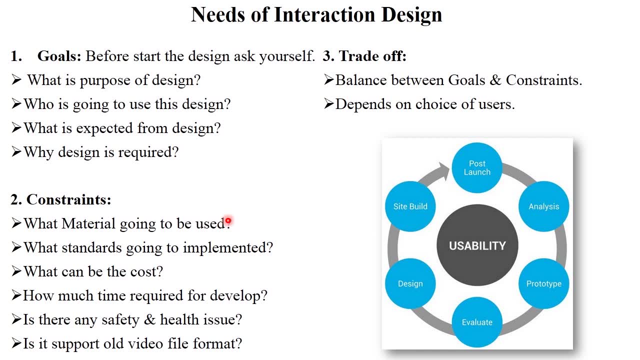 system and digital things. so all those things, or all those appliances, includes interactive designs right next. the next point is needs of interaction design. so a developer thinks so many thing about how to design a particular product, how to design a particular systems, right. so needs of design is based on three parts, that is, goals, constraints and trade-offs. 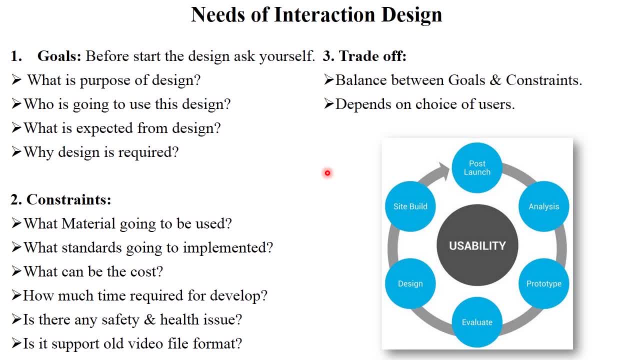 before start the designing part or before start the particular designing applications. right, the goals are: what is purpose of design? you must know about what is the purpose of design, why you design the particular product. you must know answers of all that questions. then, who is going to use this? 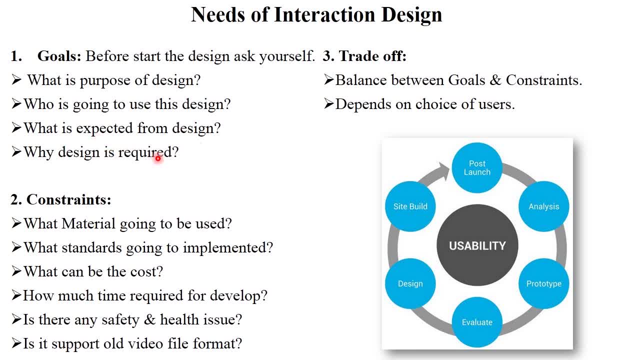 design. that is expected from design and why design is required right, for example, banking applications. so purpose of design is it's easy to handle all the customers and all the all the persons or stockholders that work there, right, who is going to use this design? all the customers of that. 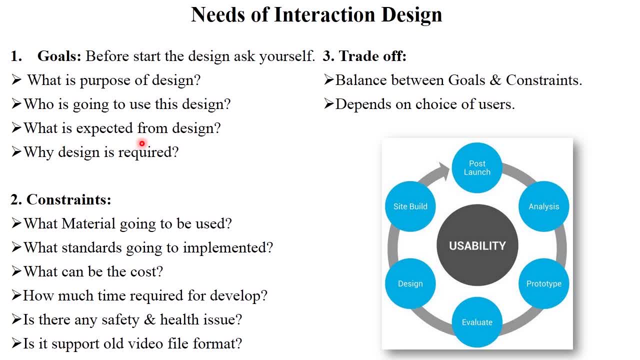 particular bank use those appliances. what is expected from design? so this design is suitable or easy to understand of each and every people, whether the peoples are technical and non-technical, and why design is required. because if you are not technical, then you are not going to be able to. 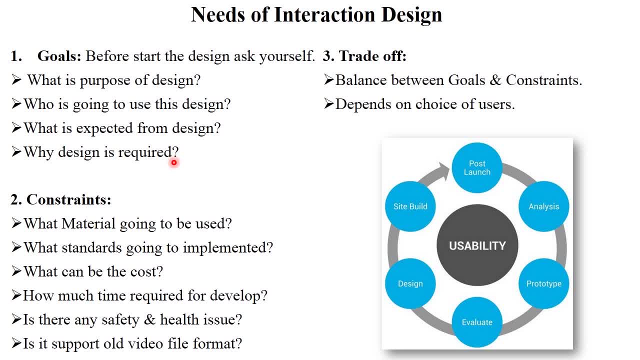 is easily provide all the services- online services as well as offline services- right, So these are the goals of that particular design. Next, constraints. Constraints means what material going to be used, what standards going to be implemented, what can be the cost, how much time required for develop. 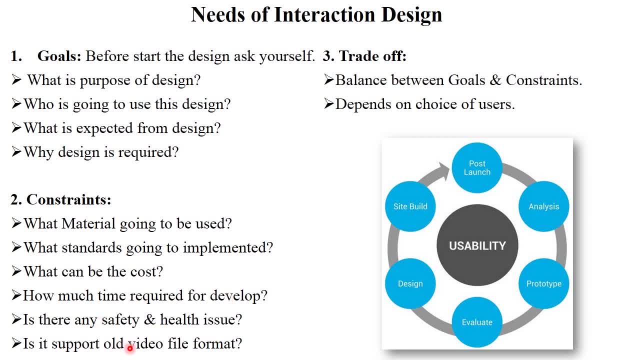 if there any safety and health issue, and is it support old video file format? Let's take one example, for example, WhatsApp Right. What material going to be used? Material simply means what types of operating system processes whether you will run that particular product right. 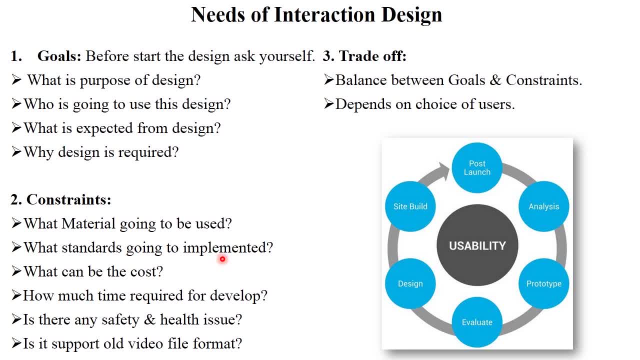 What standards going to be implemented. You know the standard of your applications right. So, for example, WhatsApp, YouTube, they have the proper design and proper interactive system. So, user attracted towards that, They have a high standard right. 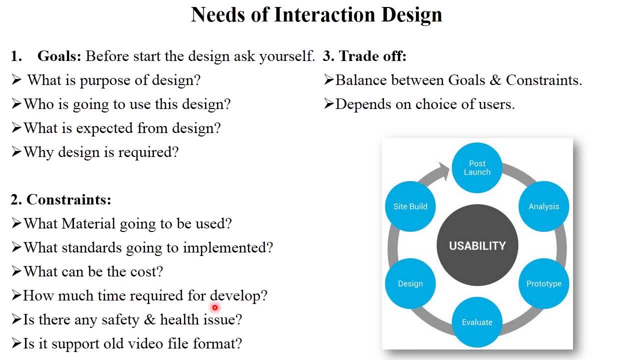 What can be the cost, How much time required for development And is there any safety and health issue? You must know about all those things, okay. So some YouTube videos supports old video file format. some applications- okay, And some applications not, support that format. 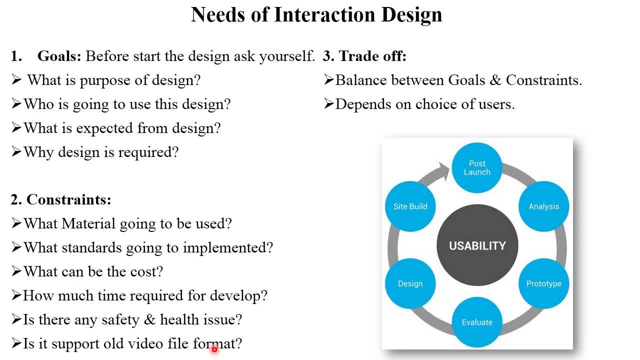 So you must remember this thing about that, okay? Or it is similar to the images. also, Some applications supports JPG format image. Some applications supports PNG format, right. So you must know, You must know all those things before start the design, right? 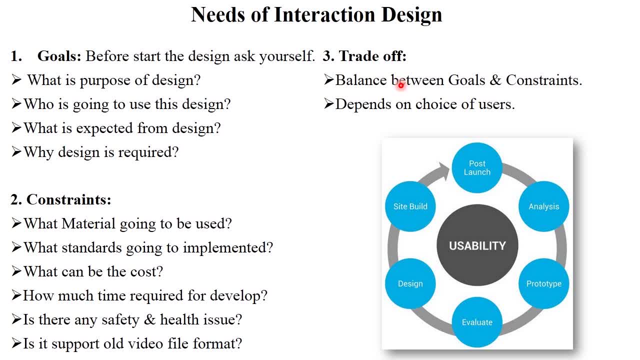 And next trade-off. Trade-off means it is a balance between goals and the constraints. okay Means proper goals and proper constraints must be followed And it depends on choice of the users, right? So these are the needs of interaction design. 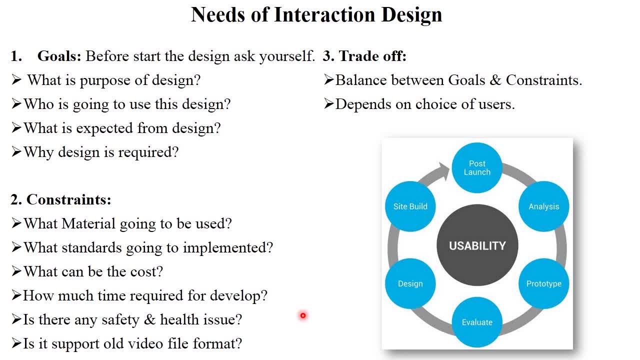 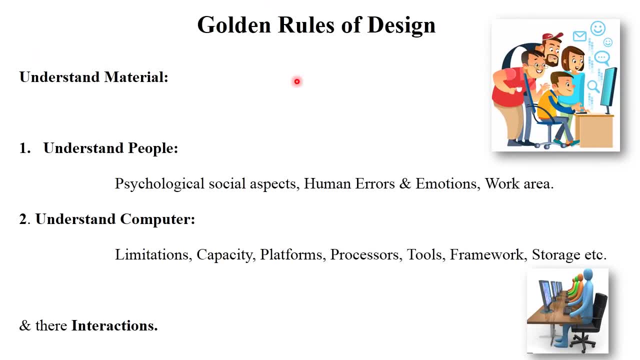 Before start the designing of particular product, particular application, you must remind all those things Clear. Next Next part is golden rules of design. Golden rules of design must involve understand material. There are two types of material, like understand people and understand computer. 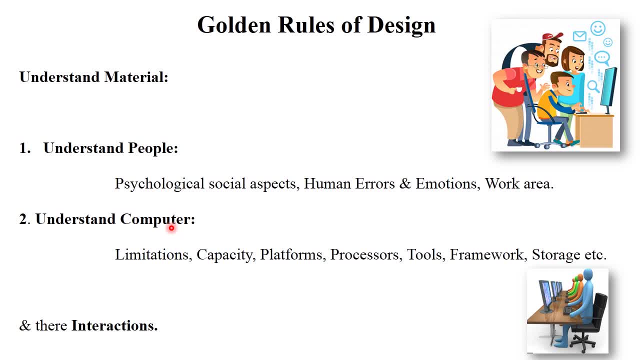 Before start the design, you must know the requirement of that particular product. okay, So understand people means to understanding psychological, social aspects, human error, emotions and also work area. There are some applications that must be used in only organization, Like a reservation system. 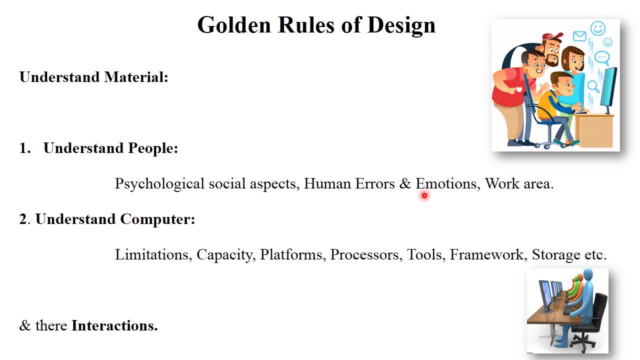 This kind of application used in airport reservation, train reservation. So each and every application has particular people and particular work area. right, You must understand all those things. And next is understand computers. Understand computers include limitations, capacity, platform processes to understand tools, framework storage, etc.